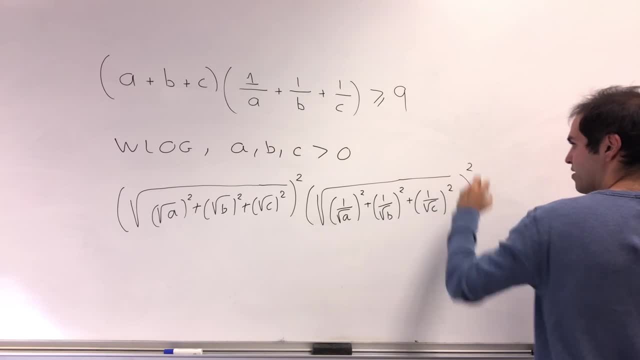 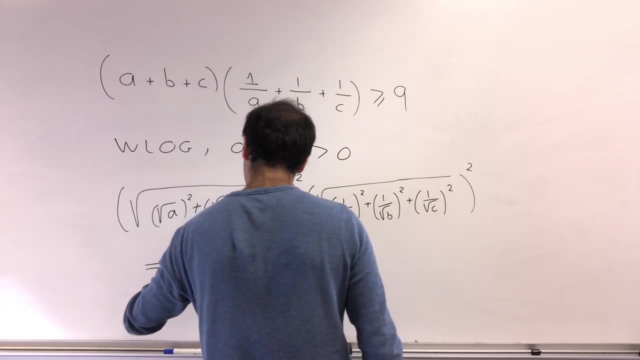 squared and you also square this. So all of this is none other than the length of u squared times the length of v squared, twice the length of c squared. So we just take all these things out and we can solve this problem by computing this. 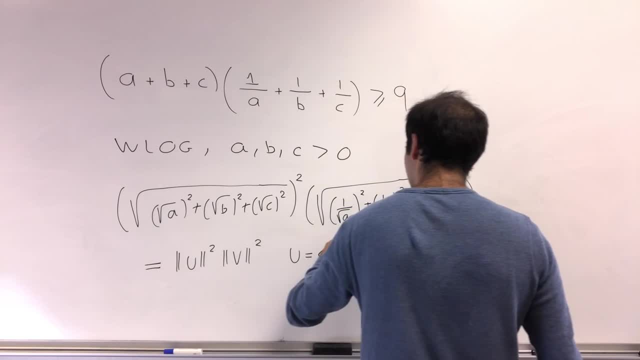 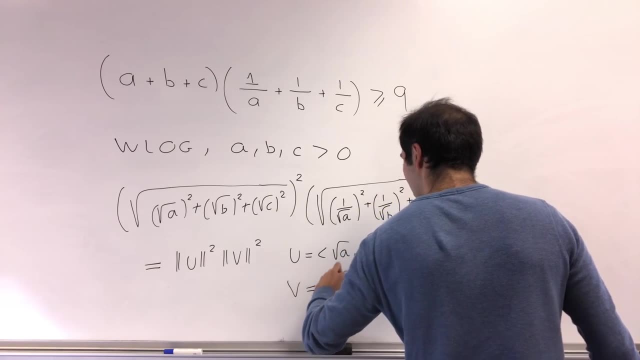 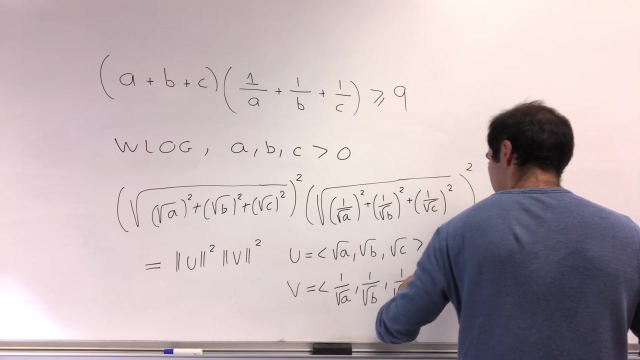 squared, where u is the vector square root of a, square root of b, square root of c, And v is the vector 1 over square root of a, 1 over square root of b, 1 over square root of c. 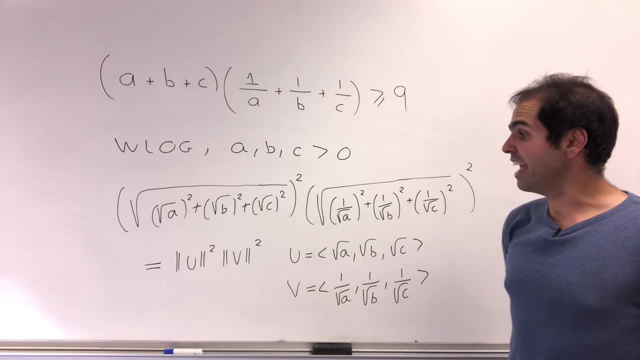 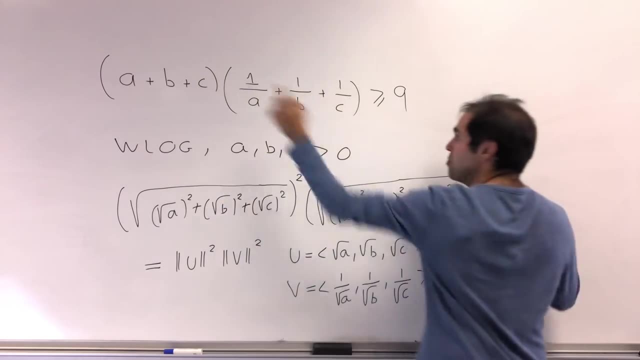 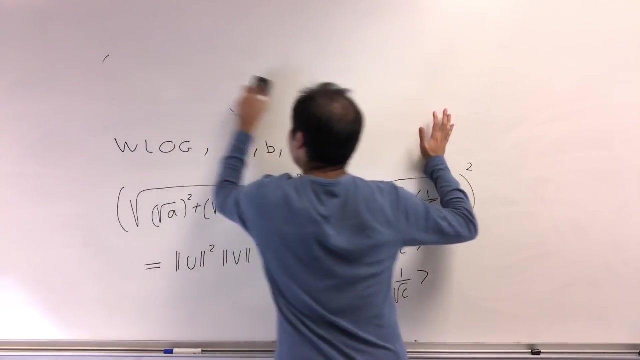 And now what we would like is some identity that relates those lengths with dot products. Because notice, if you just naively multiply all those components, you get 3.. So somehow we want this 3 to appear, But luckily there's a beautiful identity which relates dot products and lengths. 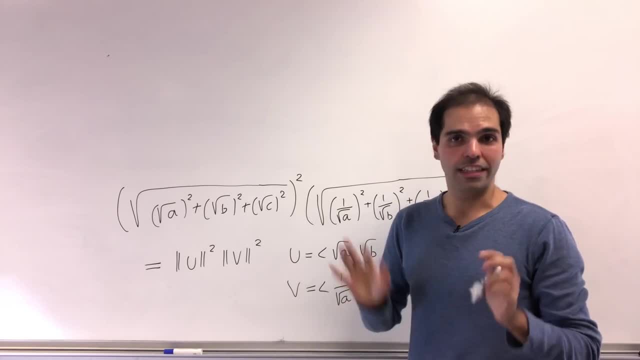 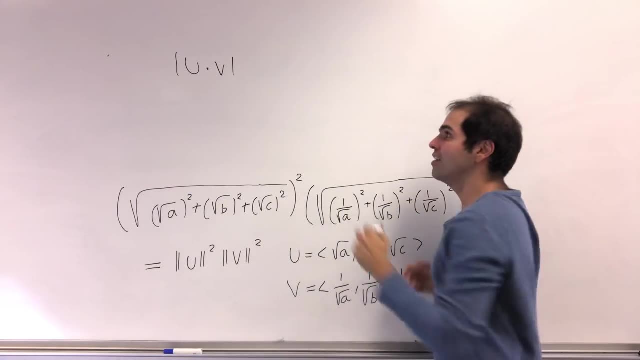 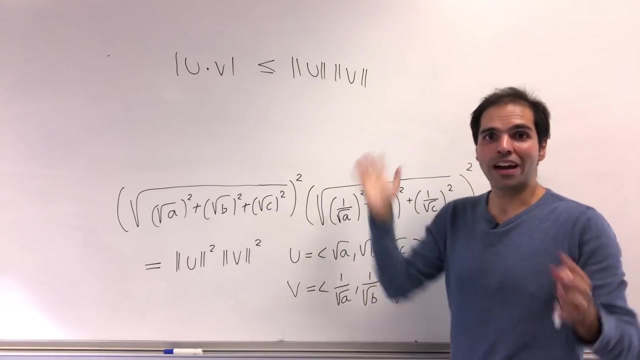 And this is called the Cauchy-Schwarz-Bunyakovsky inequality, which simply says the magnitude or the absolute value of the dot product is less than or equal to the length of u times the length of v, Which, by the way, there's a beautiful proof of this on my channel. 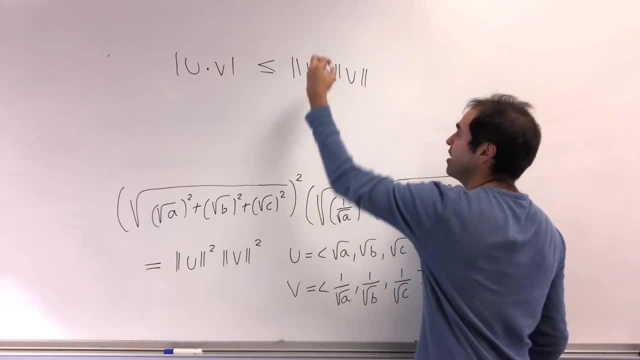 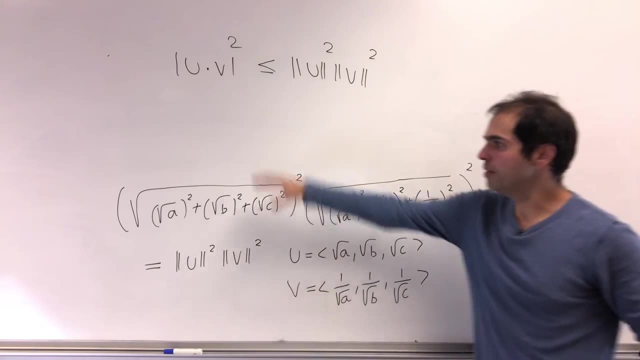 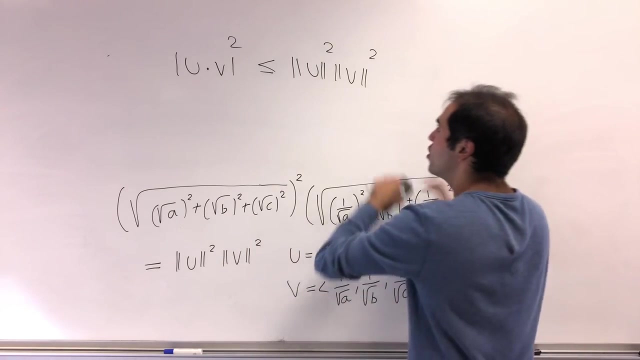 And, in particular, since we want length of u squared and length of v squared, we just square both sides. So now, going back to our problem, the quantity that we wanted is length of u squared times, length of v squared, which now becomes greater than or equal to the length of u squared times. 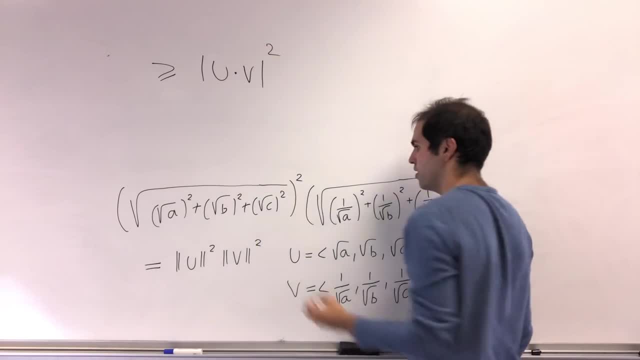 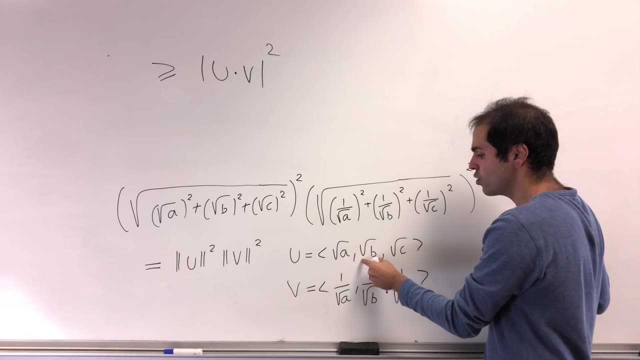 length of u dot, v squared. But now what is the dot product? Well, square root of a times 1 over square root of a, which is 1.. Square root of b times 1 over square root of b, which is 1.. 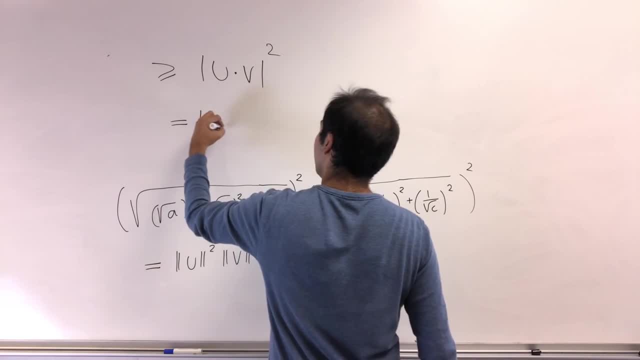 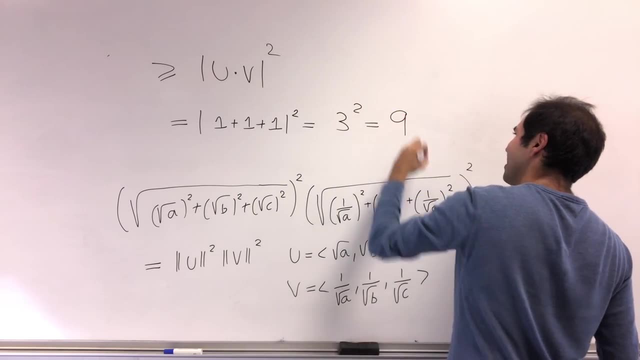 And here also 1. So what you get, is absolute value of 1 plus 1 plus 1 squared, and that's basically 3 squared, which is 9.. Nein, das gibt's doch nicht. Wir haben das Positiv nicht.